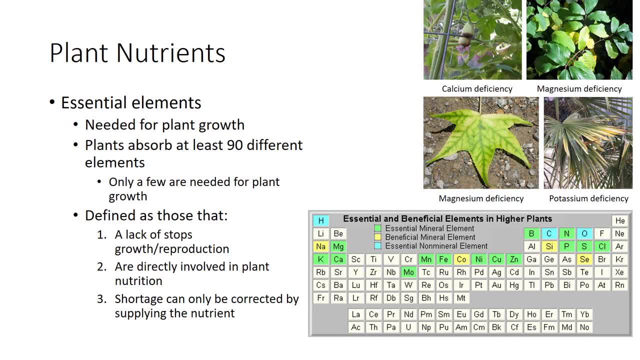 important for human and animal nutrition. Many elements are needed by neither plants nor animals, and others, like lead, are even toxic. Thus, plants contain many elements not needed for growth. Which elements are essential? The most commonly accepted rules for determining whether an element is essential are as follows. 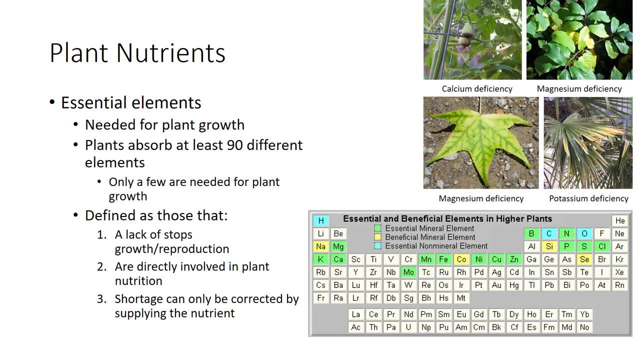 1. A lack of the element stops a plant from completing growth or reproduction. 2. The element is directly involved in plant nutrition, not merely taking up space in plant tissues. And 3. A shortage of the element can be corrected only by supplying that element. 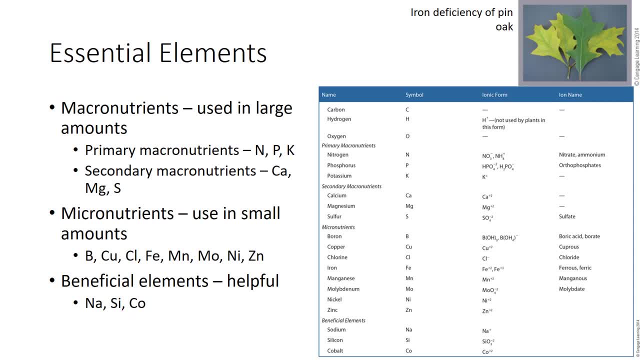 Based on these rules, 17 essential elements are identified by most scientists. Several others play a role in the nutrition of some plants but cannot yet be considered true essential elements for all plants. Some of these beneficial elements are also identified in the table. A live plant is mostly water, some 90% by weight. 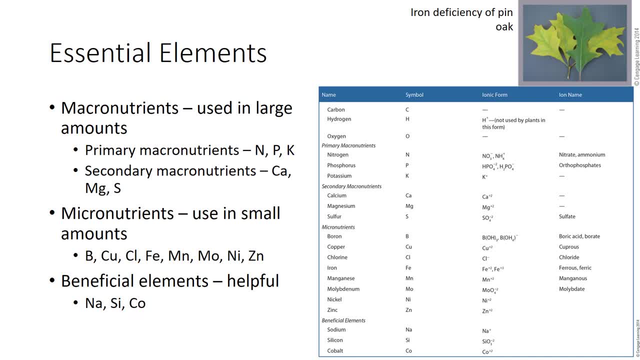 Of the remaining mass, the dry weight, most is carbon, oxygen and hydrogen in the form of organic compounds. Plants obtain these three from air and water during the process of photosynthesis. The remaining 14 elements are obtained from the soil, and we might call these mineral nutrients. 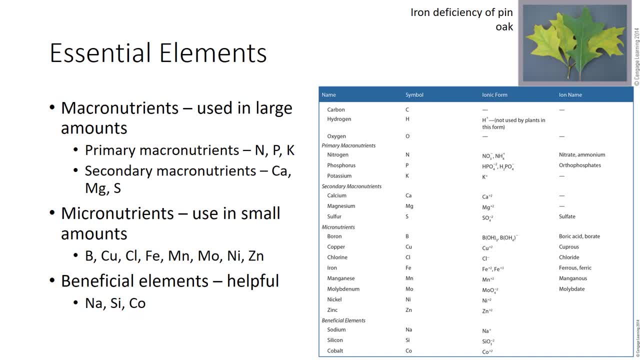 Plants use six of the 14 mineral elements in large amounts. These six macronutrients are the main nutrients. These nutrients are nitrogen, phosphorus, potassium, calcium, magnesium and sulfur. In the following relationship, the six nutrients are listed in decreasing order from the greatest. 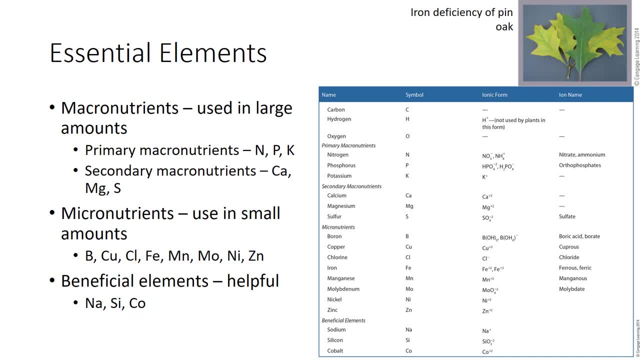 amount used by most plants: nitrogen to the smallest amount, sulfur. They are divided into primary and secondary macronutrients. The other eight nutrients listed in the table are labeled micronutrients or trace elements because they are used in small amounts. 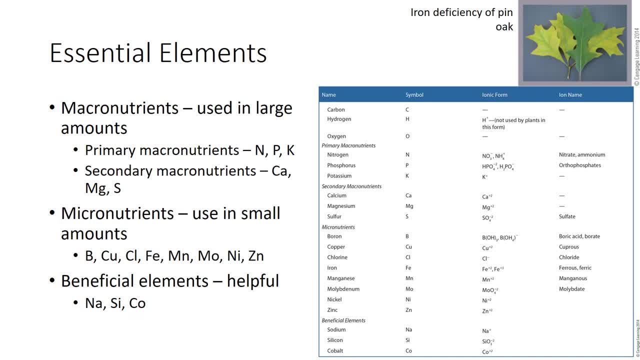 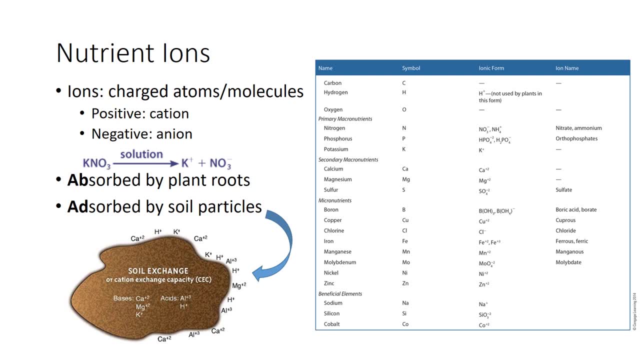 The term micronutrient does not, however, mean the elements are unimportant. Ions are charged, atoms or molecules. The charge, either positive, a cation- or negative, an anion- results when there is a difference between the number of electrons and protons. 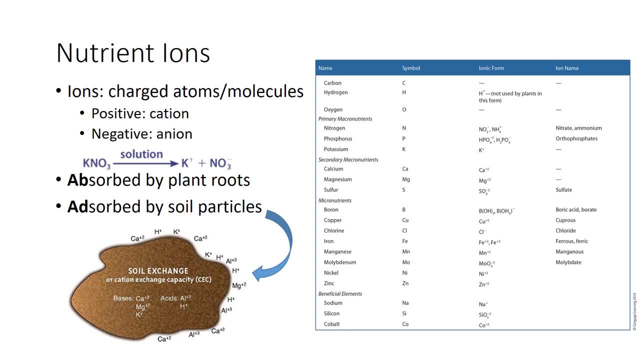 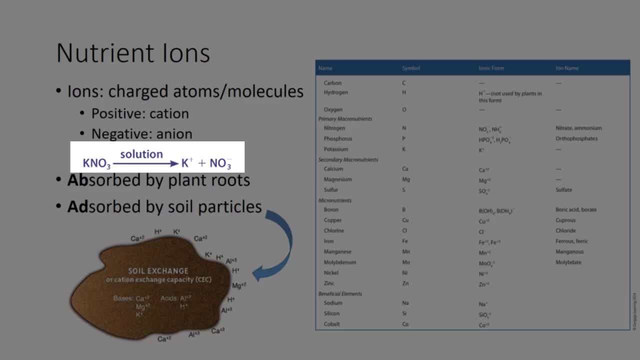 One way ions form in soil is when compounds dissolve in water. For example, when the soluble fertilizer potassium nitrate dissolves, the molecule breaks into two ions: The potassium and nitrate. ions now in solution can be absorbed by plant roots. 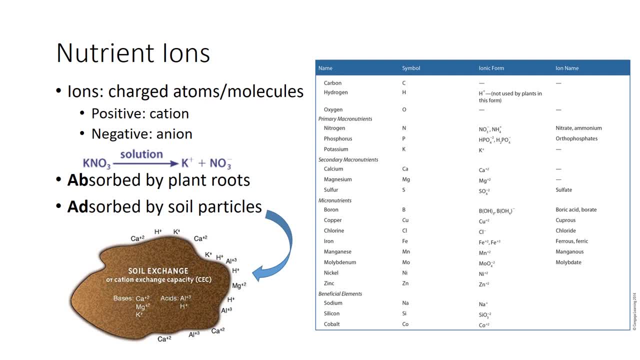 The concept of nutrients as ions is important. The concept of nutrients as ions is important. Plant roots absorb nutrient ions. soil particles adsorb them. Absorb means to take in something like a sponge absorbing water. Adsorb means to attract a thin layer of molecules to a surface where they stick. 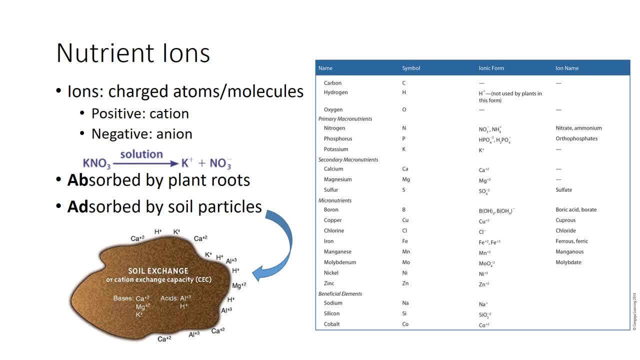 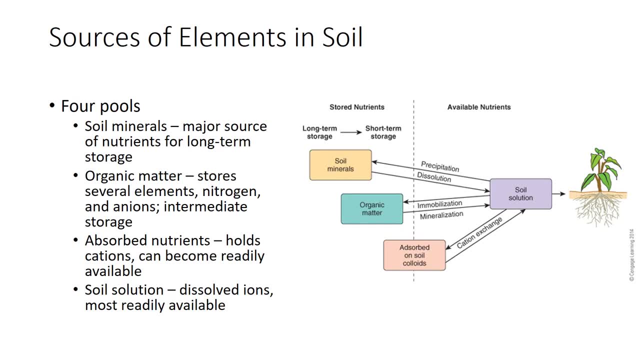 The table shown lists each nutrient in the ionic forms most commonly absorbed by plants. Any special name for the ion is also listed. Nutrient elements are present in the soil in four forms. Together, these four pools perform two functions: to store nutrients and to make them available. 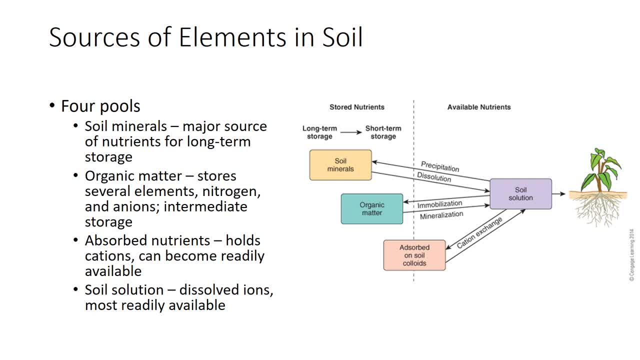 to plants. Minerals are the major source of all soil-supplied nutrients except nitrogen. Soil minerals are the longest-term storage. Weathering frees the elements slowly over time, dissolving the minerals into ions. Organic matter stores large amounts of several elements like nitrogen and the nutrient anions. 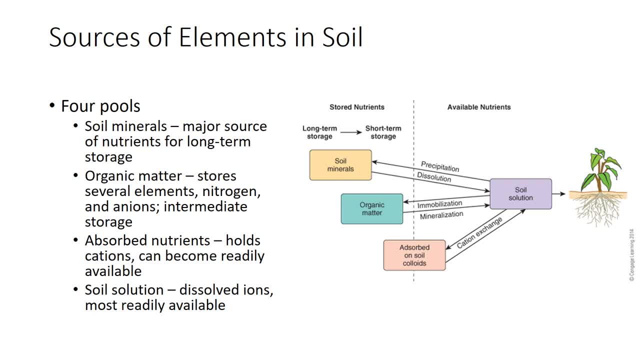 Organic matter is an intermediate to long-term form of storage. Since elements are stored in the soil, they can be stored in the soil for a long time. They are freed for plant use by decay. Some nutrients in fresh organic matter are released fairly quickly, while those in humus. 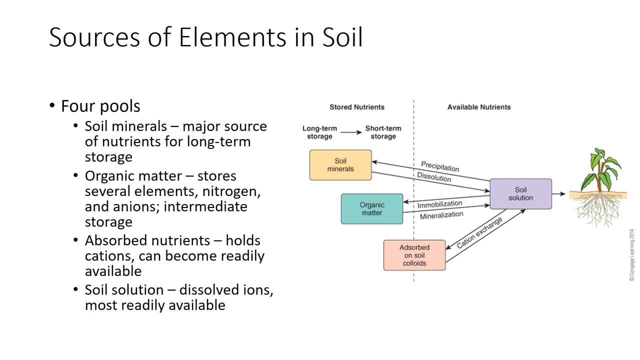 are released more slowly. Adsorbed nutrients are held in the soil, attracted to clay and humus particles. Adsorption occurs because clay and humus particles are negatively charged. Many plant nutrients are positively charged and so stick to the soil particles. Adsorbed nutrients are held fairly tightly by particles, but most become readily available. 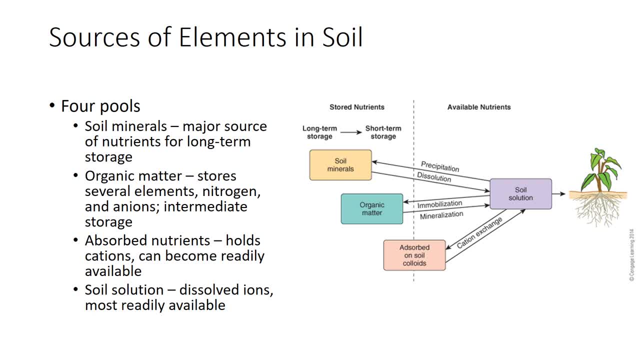 to plants. Nitrogen ions dissolved in soil water are the most readily available form of nutrients. The mixture of ions in soil water is termed the soil solution. Plants absorb ions directly from the soil solution. However, these nutrients may be rapidly consumed or leached away by percolating water. 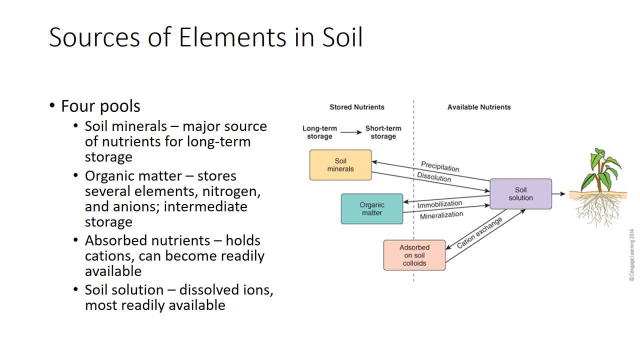 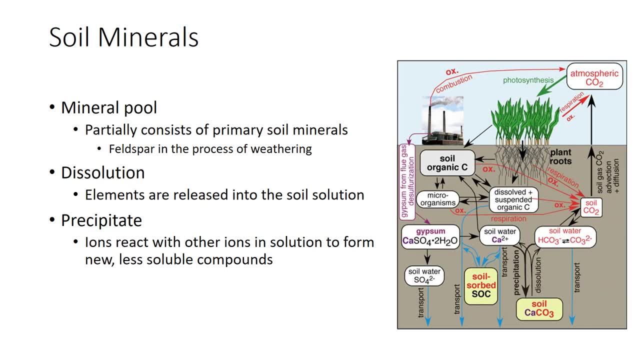 As plants withdraw nutrients from the soil solution, elements held in reserve can become available to plants. While nutrients are held in reserve, they are protected from leaching and other losses. The mineral pool partially consists of primary soil minerals. The soil is rich in nitrogen and nitrogen. 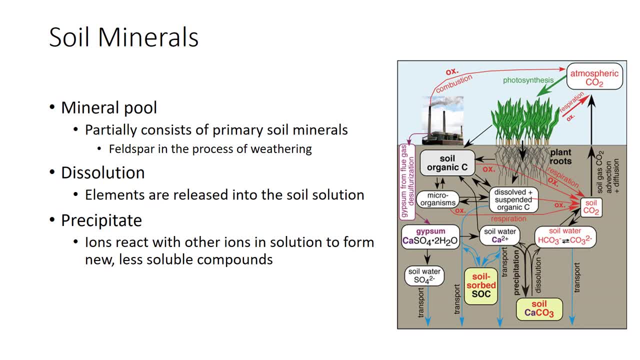 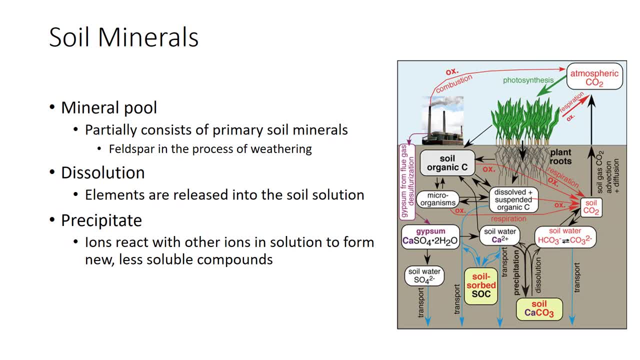 Dissolution may proceed very slowly in the case of weathering-resistant rocks like granite, and more quickly in other rocks like limestone. Ions of nutrient elements can react with other ions in solution to form new, less soluble compounds. These new compounds precipitate out as solid particles of new or secondary minerals that. 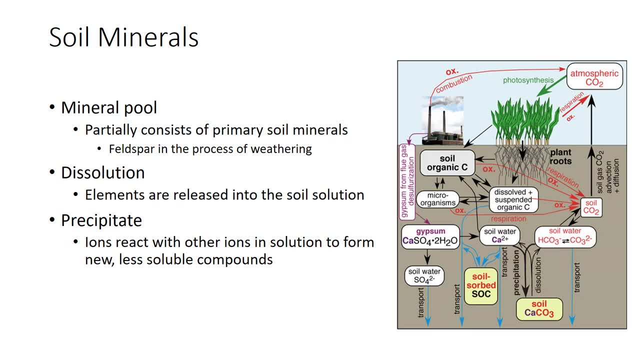 form in the soil. These reactions strongly reduce availability of some nutrients. in many soils, The products of precipitation are themselves subject to dissolution and may later re-enter the soil's solution. Nutrients are adsorbed on soil, colloids, tiny clay and humus particles that carry a slight 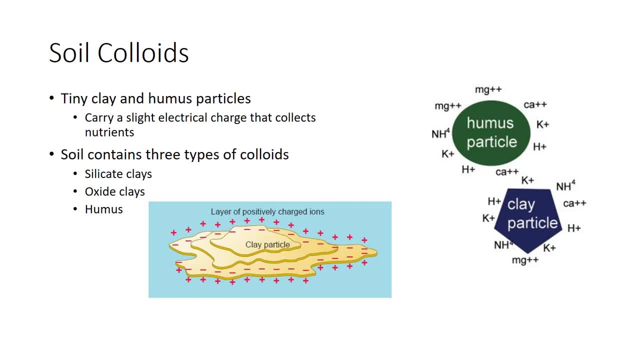 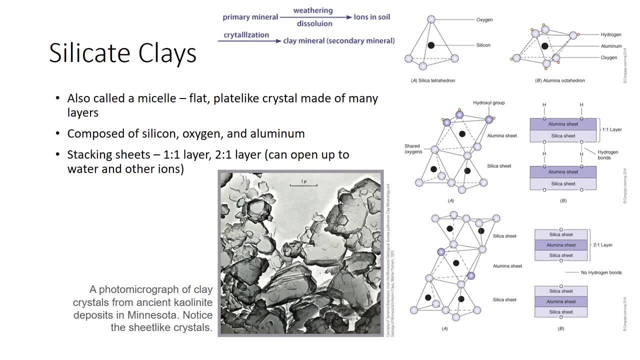 electrical charge. This charge is important because it attracts nutrient ions. The soil contains three types of colloids: silicate clays, oxide clays and humus. Clay minerals are not simply pieces of silt or sand broken into tinier particles. 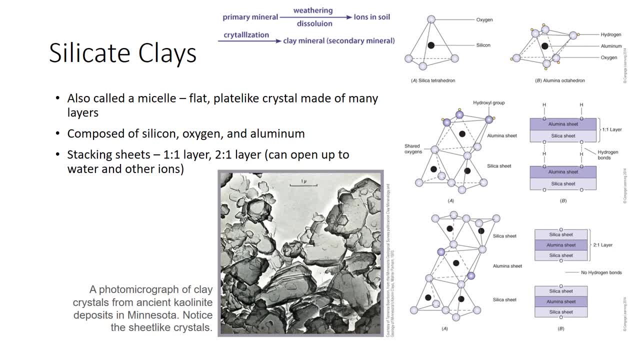 A clay particle is a tiny crystal of mineral formed in the soil from the weathered products of minerals like feldspar or mica. Feldspar and many others are primary minerals of the earth's crust, while the clay minerals that form from the products of their weathering are called secondary silicate minerals. as 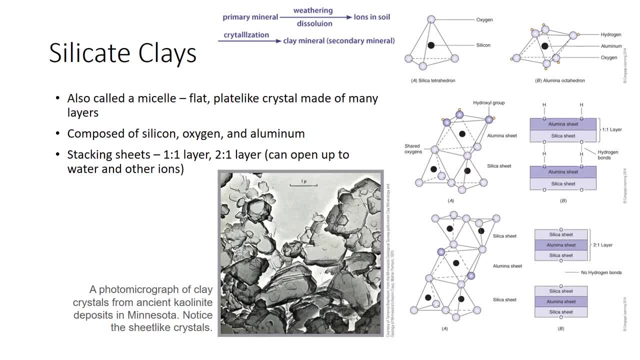 shown in the process equation, A particle of silicate clay called a micelle is a flat, plate-like crystal made of many layers. Each layer in turn is made of two or three sheets. The sheets are mainly composed of three elements: silicon, oxygen and aluminum. 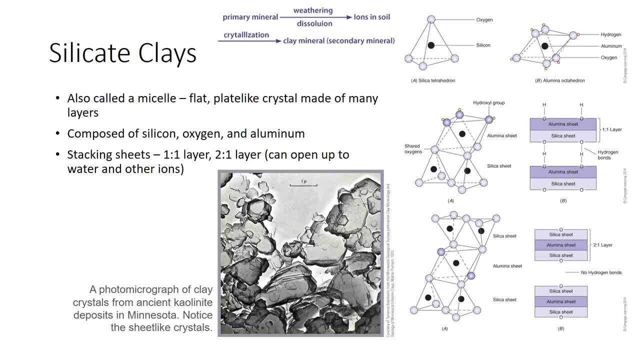 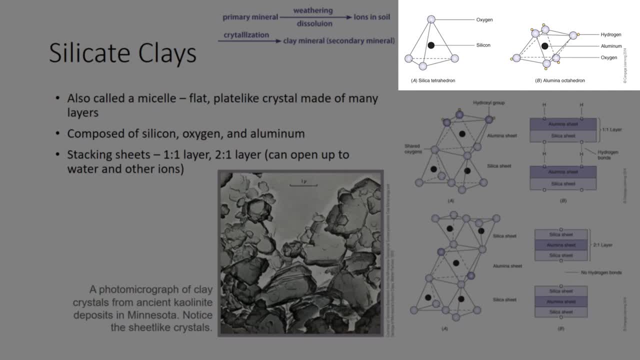 These three elements combine to form several kinds of sheets which can combine to form several kinds of clays In the soil. silicon combines with oxygen to form the silica sheet. The second important sheet in silica clays is the alumina sheet, which has aluminum in. 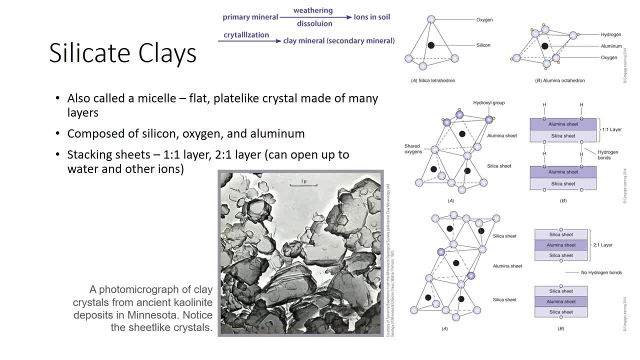 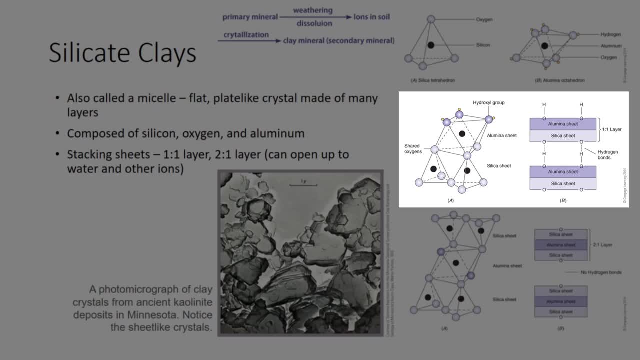 the center surrounded by hydroxyl groups. These sheets can stack atop one another in several ways to form a complete clay crystal. The simplest stacking joins a single alumina sheet to one silica sheet, forming what is called a one-to-one layer. Two layers can now join by hydrogen bonding. 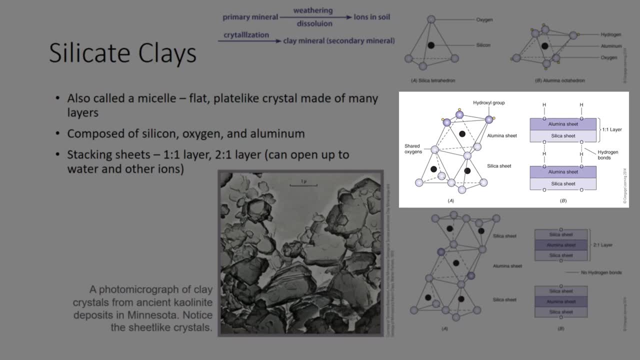 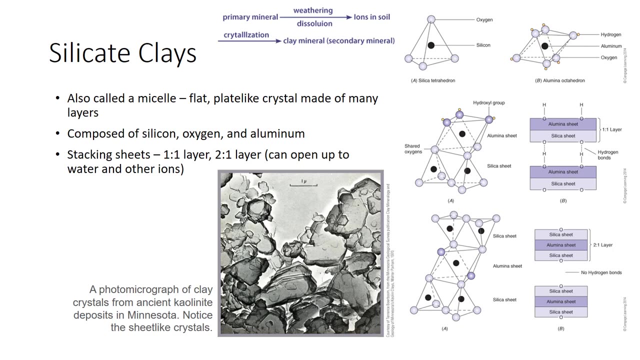 The hydroxyl groups of one layer bond to the oxygen atoms of another. Hydrogen bonds hold the layers in the clay crystal together tightly. One clay mineral composed of one-to-one layers is kaolinite. A second way to stack sheets is to sandwich an alumina sheet between two silica sheets. 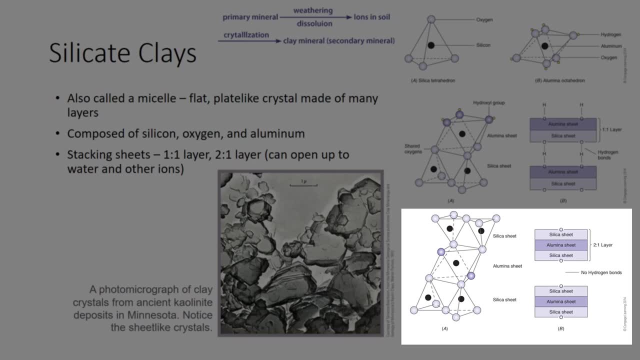 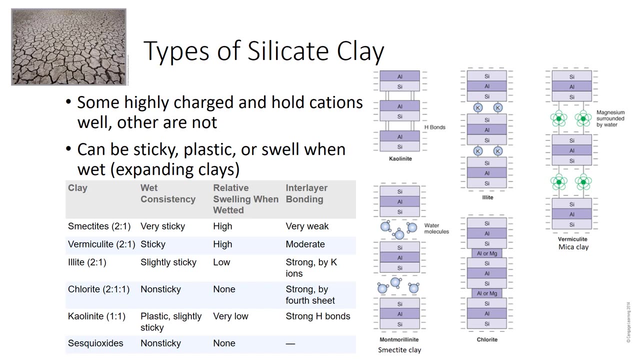 This is a two-to-one layer. This is a two-to-one structure. The bond that holds the layers together are much looser than hydrogen bonds, so most two-to-one clays can open up. So why am I telling you this? Several types of clays result from the ways in which one-to-one or two-to-one layers bond. 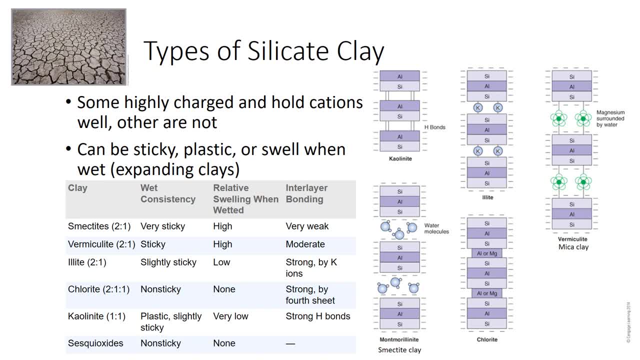 together. Some clays are highly charged and hold cations well, Others are not. Some clays are sticky, Some are plastic And some swell when wet. Two important traits of silica clays depend on how easily the layers can be separated. 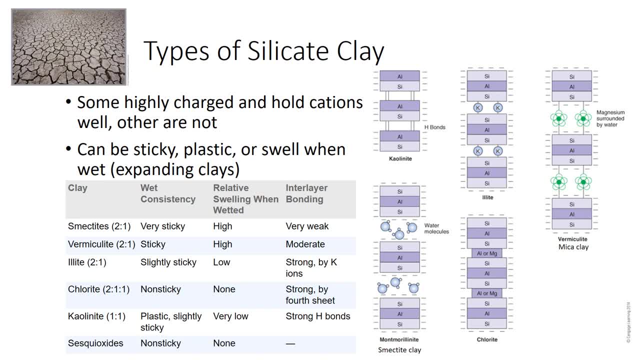 If they loosen easily, They can enter the micelle between the layers and the particle will swell when wetted and shrink when dried. Such clays are called expanding clays. If layers separate, more surface area is exposed for adsorption of cations. 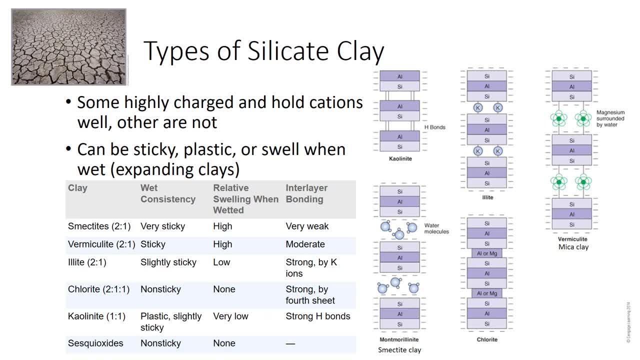 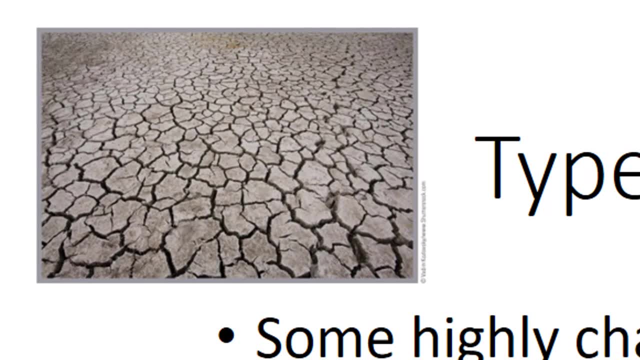 Thus, clays with loosely bound layers usually hold more nutrients. Notice the mud cracks in this expanding clay. This vertisol swells as it wets and shrinks as it dries, forming these deep, wide cracks. You can see the amount of stickiness and swelling for different types of clays in the table. 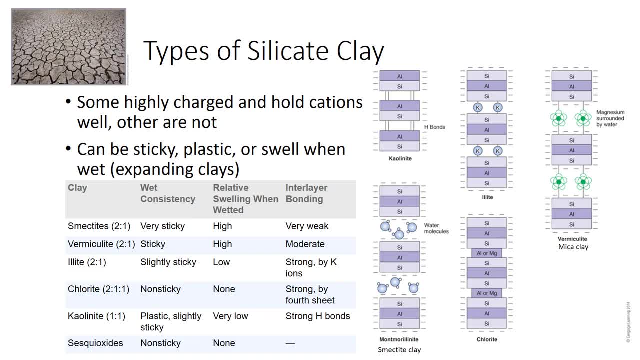 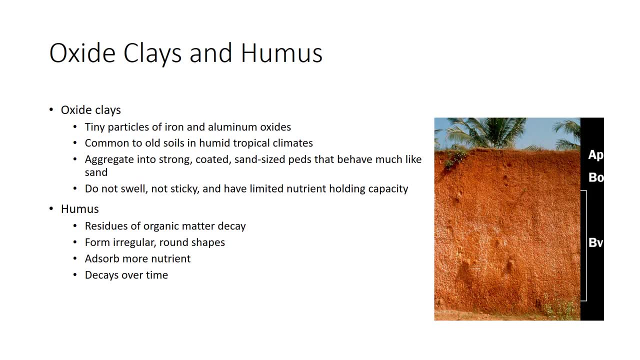 Vermiculite, The most commonly used in potting mixes, is chosen because it has high nutrient-holding capacity. Oxide clays, called sesquioxides, are tiny particles of iron and aluminum oxides. Oxides are common to old soils in humid tropical climates. 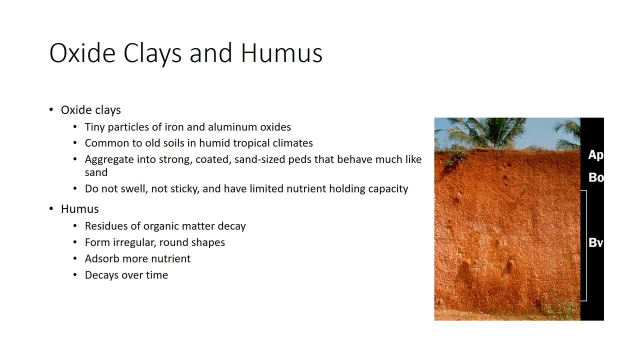 Long periods of weathering leach out silica and some alumina, leaving behind the oxides. Oxide clays tend to aggregate into strong coated, sand-sized pads that behave much like sand. Oxide clays can form stacked sheets, but do not form their crystals. 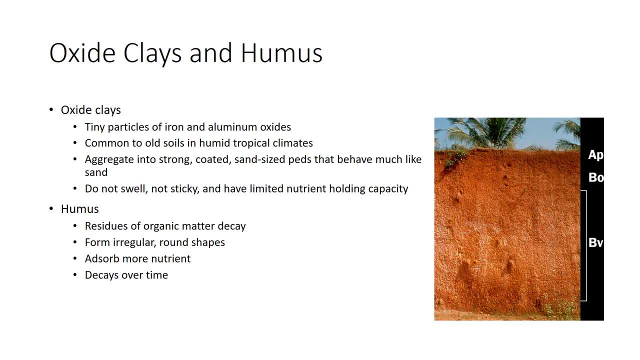 They are not very flexible. They have a crystalline structure of silicate clays. Oxide clays do not swell, are not sticky and have limited power to hold nutrients. Oxide clays are typical of oxosol soils and the red color often found in oxosols reflects. 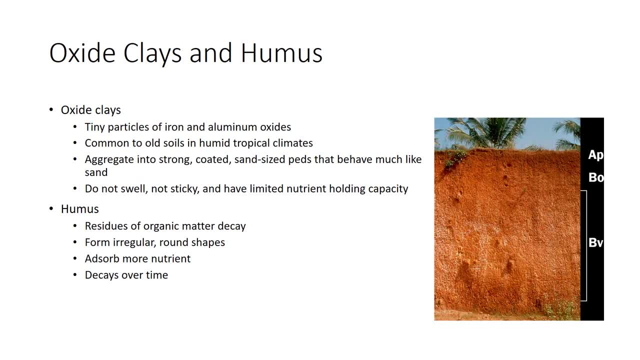 the reddish hues of iron oxides. Hemis particles are the residues of organic matter decay. They are not crystalline and form irregular round shapes. They have none of the physical properties of clays, like stickiness or plasticity. However, they have more power to absorb nutrients. 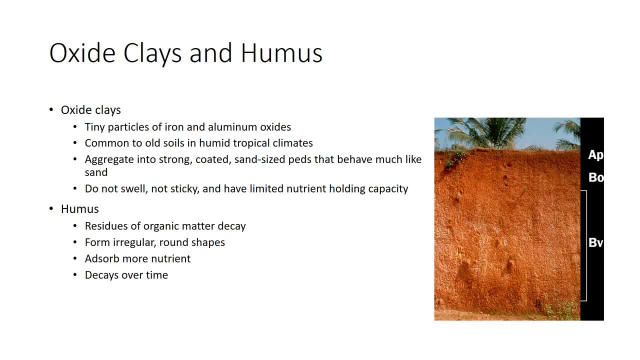 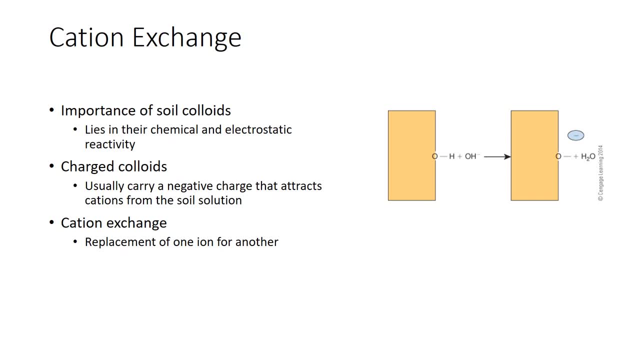 They absorb nutrients than clays. Hemis is not stable. It decays over time to carbon dioxide. The importance of soil colloids lies in their chemical and electrostatic reactivity. Their electrically charged surfaces are able to attract and absorb a wide range of ions. 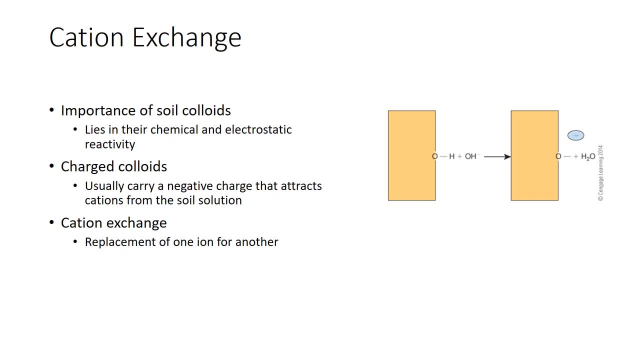 and molecules in the soil. Most important here are plant nutrients, but also materials like pesticides and a variety of other organic molecules. These activities profoundly influence soils and how we manage them. Soil colloids: 3. A negative charge that attracts cations from the soil's solution. 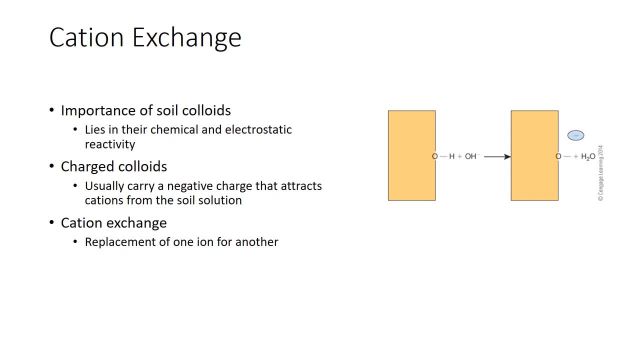 Clay particles gain a negative charge in two ways. First, the loss of a hydrogen ion from a hydroxyl group on the surface of a clay micelle leaves oxygen with a negative charge that can attract cations from the soil's solution. The second process is isomorphous substitution. 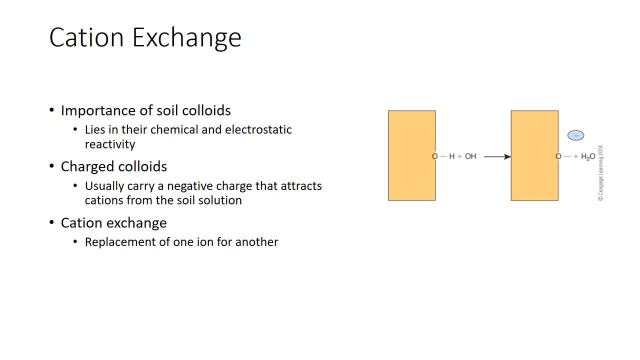 One cation can replace another cation of similar size in a clay sheet. For instance, aluminum can replace one cation of similar size in a clay sheet. For instance, aluminum can replace a normal cation of similar size in a clean sheet. 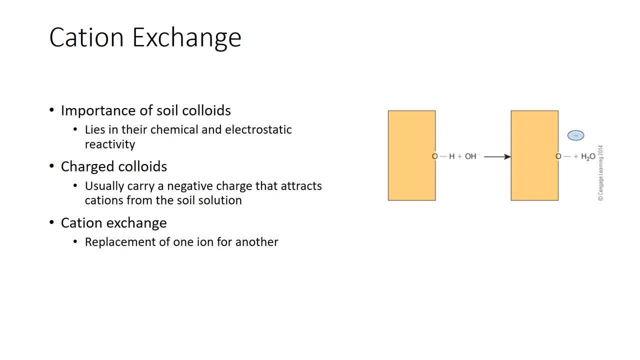 3 can replace a silicon atom- Si plus 4, in a silica layer. While the cation fits, it has a smaller positive charge. This leaves a spot in the crystal that is short of positive charges. These spots acquire a negative charge Because a clay crystal contains many of these. 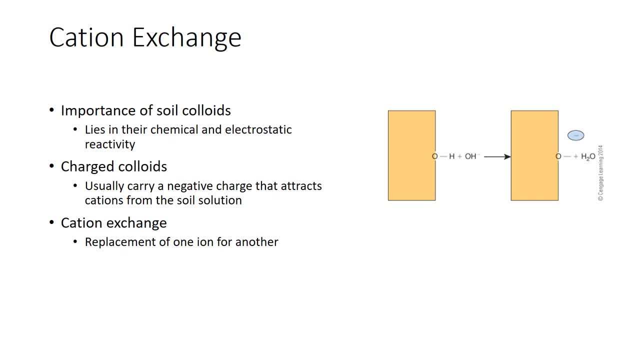 negative spots, the entire particle maintains a negative charge. The minus charge creates an electrostatic attraction for positively charged cations, so the micelle is surrounded by a swarm of cations absorbed to the surface of the clay particle. The minus and plus charges. 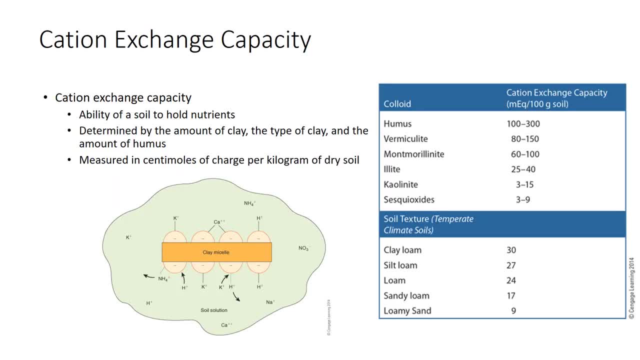 balance for a net zero charge. The negatively charged surface of soil colloids play a key role in the way nutrients behave in soil. The colloid surface is negatively charged, so it absorbs cations. Cations are exchangeable, in that if one leaves, another takes its place. The ability of a soil to 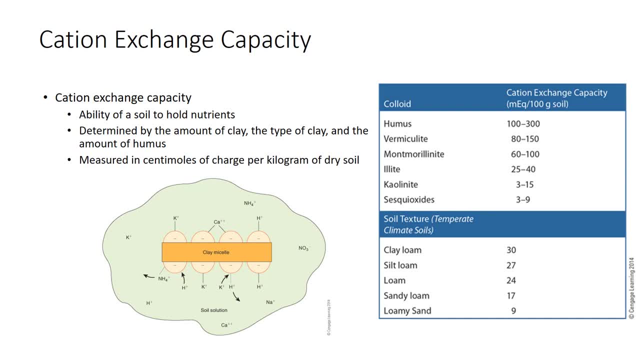 hold nutrients relates to the number of cations it can attract to soil colloids. This value, determined by the amount of clay, the type of clay and the amount of humus, is measured by cation exchange capacity, CEC, measured in centimoles of charge per kilogram of dry. 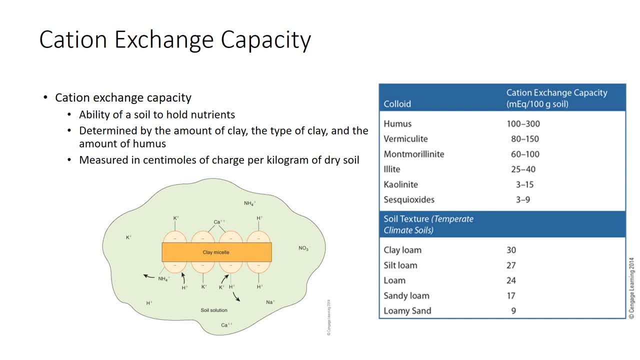 soil. It may also be expressed as milligram equivalents per 100 grams of soil. The table lists CEC values for several clays, humus and soil textures. Note that humus has a much higher CEC than clay. However, clay usually adds more CEC to a soil than does humus, because 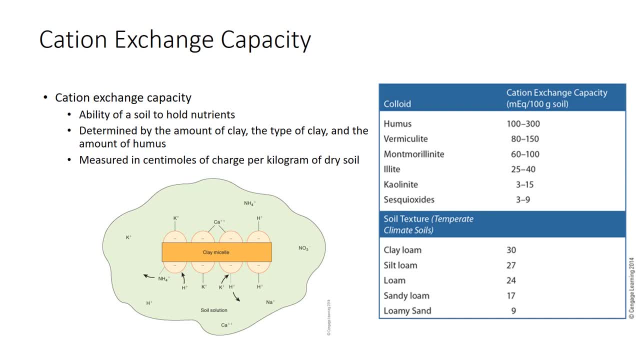 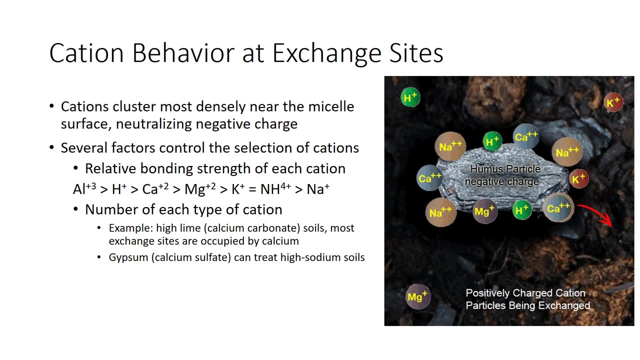 there is so much more clay than humus in most soils. Sandy soils low in clay may also gain a large portion of their exchange capacity from humus, which largely explains why the addition of organic matter is so beneficial to sandy soils. Cations cluster most densely near the micelle surface, neutralizing negative charge Cations. 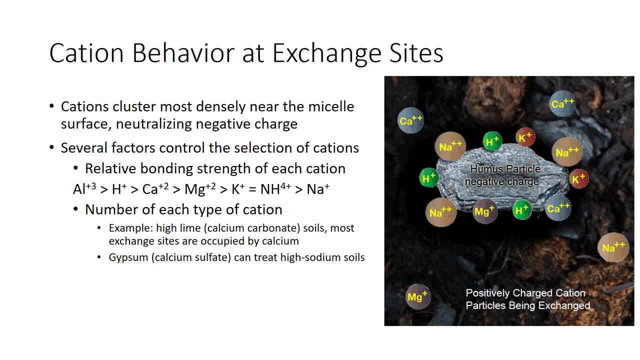 can move on the micelle and trade places or exchange with cations in solution. Several factors control the selection of cations that leave the micelle or become adsorbed. Two important factors are the relative bonding strength of each cation. Cations can be used. to control the selection of cations that leave the micelle or become adsorbed. Two important factors are the relative bonding strength of each cation. Cations can be used to control the selection of cations that leave the micelle or become adsorbed. Two important factors. 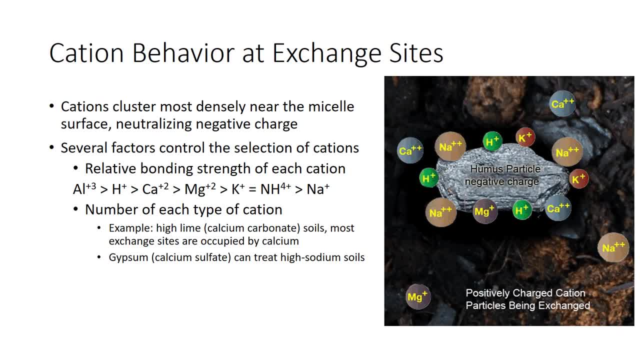 can be used to control rotation and stronger bonding freebase and Fans. interestingly on, the micelle Sodium tends to leach out of the soil's solution. The second controlling factor is mass action. Mass action means that the greater the number 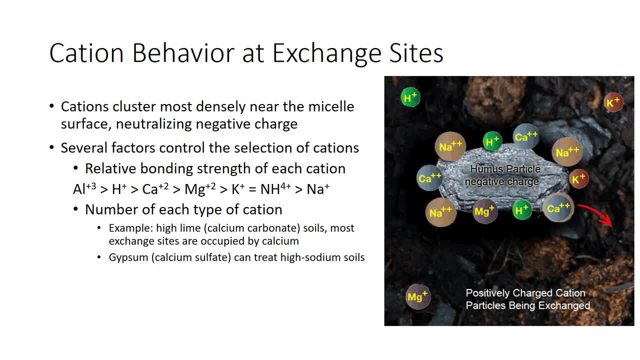 of an ion in the soil, the more exchange sites it will occupy. As an example, on high-lime calcium carbonate soils, most exchange sites are occupied by calcium. Consider treatment of high-sodium soils with gypsum. In a high-sodium soil, many exchange sites 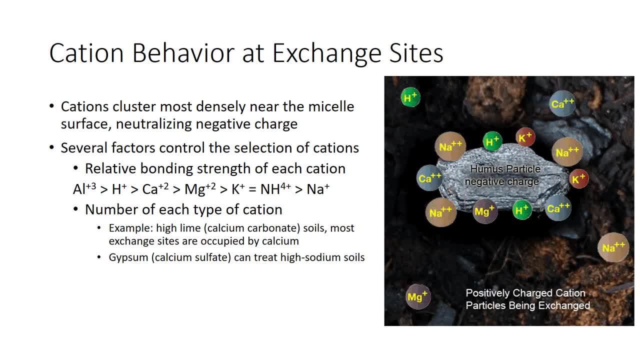 are taken up by sodium. When gypsum is added, calcium displaces sodium on the exchange sites. Displaced sodium enters the soil's solution and is leached away by heavy watering. Calcium replaces sodium on the exchange sites by means of mass action. There are more calcium ions in the solution and because calcium is adsorbed more strongly. 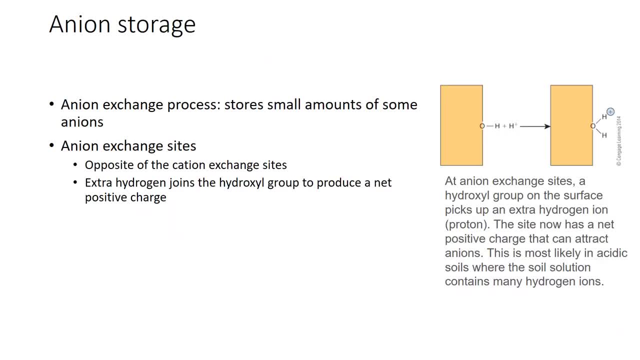 than sodium. Several nutrients are available to plants as negatively charged ions or anions. The negative charge means that an anion is repelled from a cation exchange site. While these elements, like sulfur, are to a large degree stored as organic forms in humus, an anion exchange process stores small amounts. 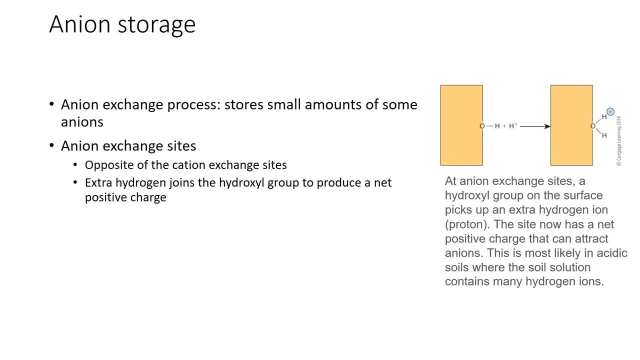 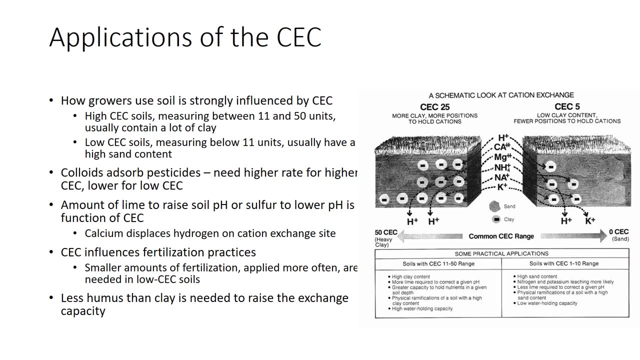 of some anions. At anion exchange sites, a hydroxyl group on the surface picks up an extra hydrogen ion. The site now has a net positive charge that can attract anions. This is most likely in acidic soils where the soil solution contains many hydrogen ions. 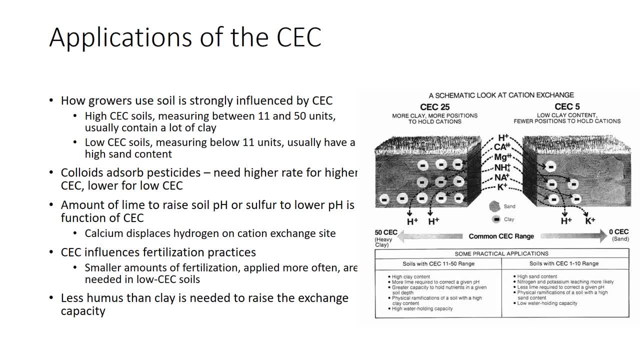 How Growers Use Soil. Soil is strongly influenced by CEC. High CEC soils measuring between 11 and 50 units usually contain a lot of clay. Low CEC soils measuring below 11 units usually have a high sand content. Sticky soils are high in the types of clays having the highest CEC. CEC. 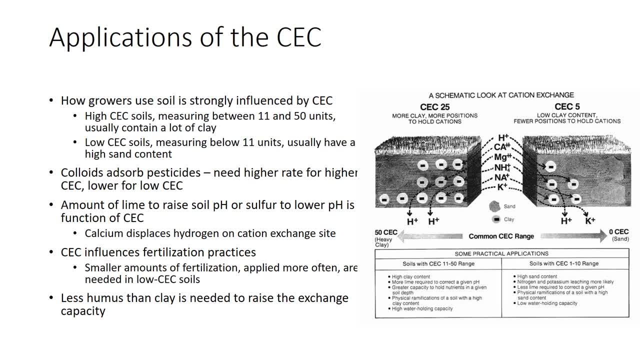 is one of the factors that determines how much herbicide should be spread on the soil. Colloids absorb pesticides as well as nutrients. Therefore, clay and humus tend to tie up many chemicals. Growers often have to apply higher chemical rates to high CEC clay soils than low CEC sandy. 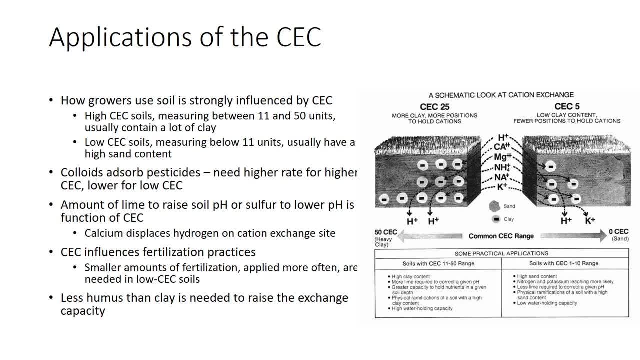 soils. On sandy soils one must be more cautious to apply a pesticide at a lower rate to avoid toxicities. The amount of lime needed to raise soil pH or sulfur to lower soil pH is also a function of CEC. In the process of liming soil, calcium displaces hydrogen on cation. 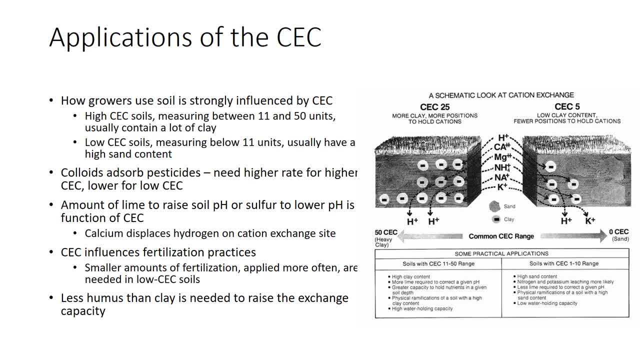 exchange sites. The more exchange sites in the soil, the more lime is needed. Therefore, growers apply much more lime to correct the acidity on food. How Growers Use Soil: CEC soils are more prone to adding more carbon dioxide to fine-textured soils than they do. 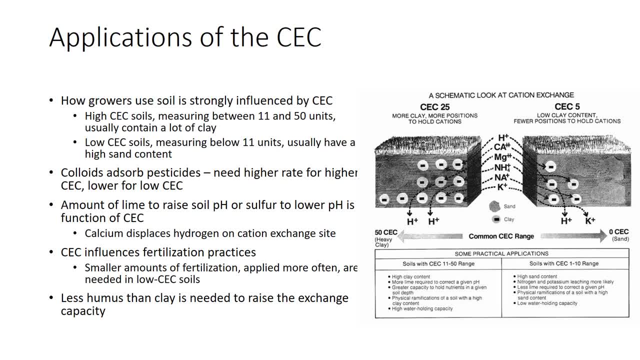 to correct coarse-textured soils. CEC influences fertilization practices. High CEC soils have greater potential to hold cationic nutrients than low CEC media. Smaller amounts of fertilizer applied more often are needed in low CEC soils to prevent leaching losses, while larger amounts 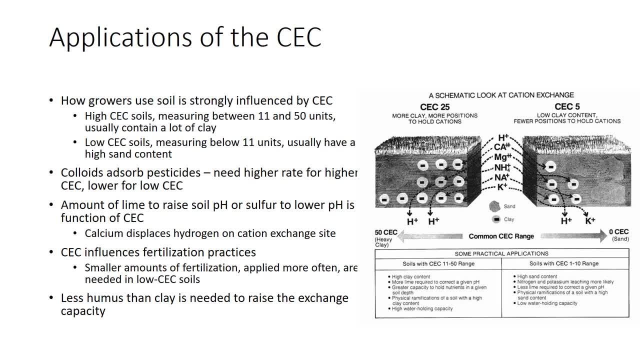 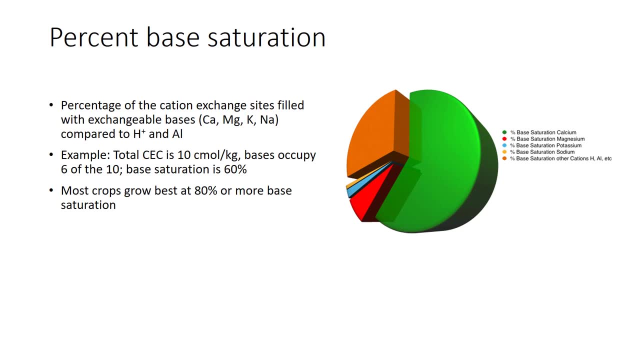 may be applied less frequently in high CEC soils. The concept of cation exchange suggests that it is easier to improve the CEC of a sandy soil by improving the organic matter content than by adding clay. Soil fertility is influenced not only by CEC- how many cations it can store- but also by 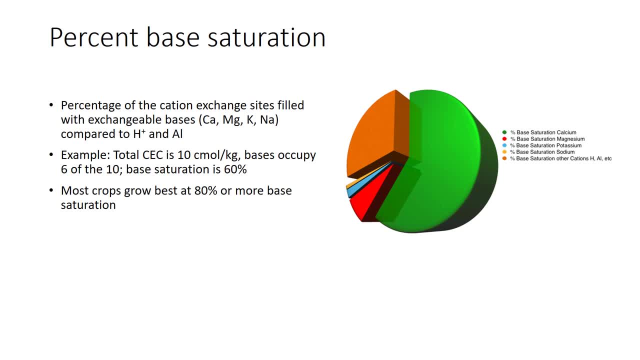 how much of the CEC is actually filled with plant nutrients? Exchange sites may be filled by members of two groups of cations. One group consists of hydrogen and aluminum, which are not plant nutrients at all. Their primary contribution is to acidify the soil. The other 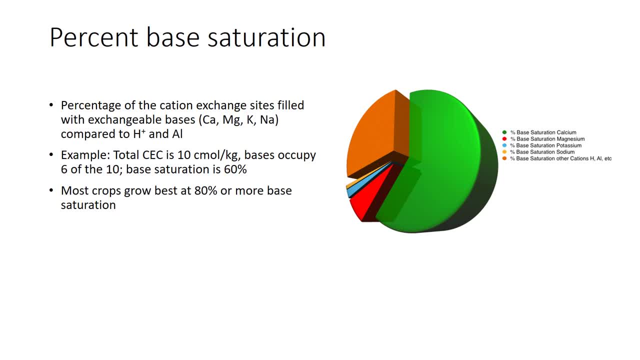 cations are called exchangeable bases and include elements such as calcium, magnesium, potassium and sodium. Except for sodium, the base of the base is nitrogen. Calcium kind of holds the hydroxyl and potassium. Soil needs a lot of oxygen to store its essential sitten. 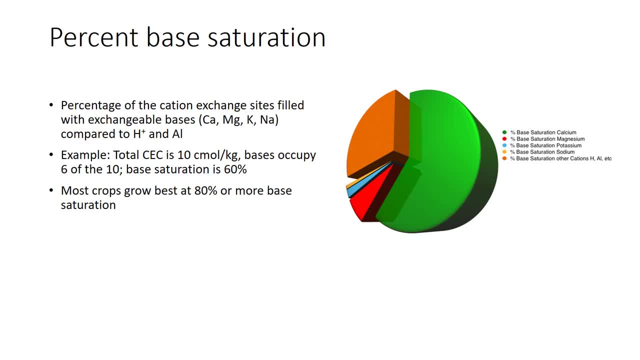 bases are plant nutrients. The percentage of the cation exchange sites filled with exchangeable bases is called the base saturation. It expresses how much of a soil's potential fertility, the CEC, holds exchangeable bases. For example, if the total CEC of a soil is 10 cMol per. 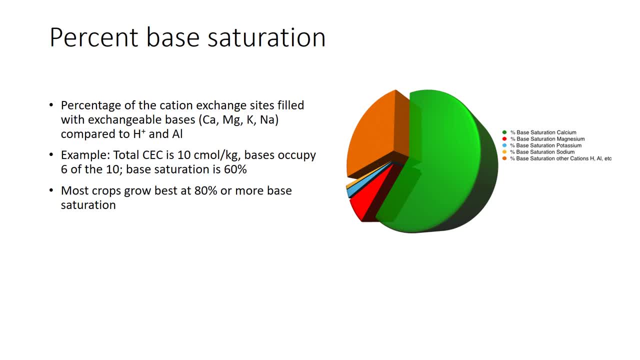 kg and bases occupy 6 of the 10,, then the base saturation percentage is 60%. Most crops grow best at a base saturation of 80% or more. These plants require a good supply of nutrients. Some trees that grow on infertile soils do well at a base saturation of about 50%. 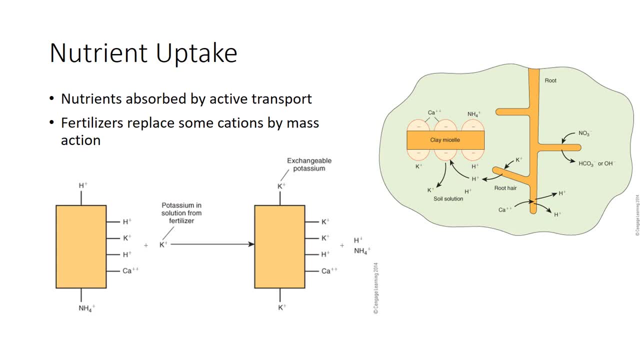 How do plants take up nutrients from the soil? Roots absorb nutrient ions from the soil solution. Roots actively transport nutrient ions through the root cell membranes, an active process that uses energy, Because roots produce energy by respiration. conditions that limit root cell respiration, like a waterlogged soil, also limit nutrient uptake. 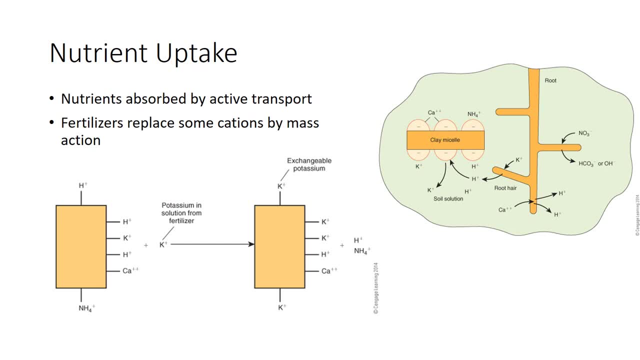 To maintain electrical balance, roots release a different ion of the same charge into the rhizosphere. For cations, a hydrogen ion is released. A loss of bases in the soil solution and a buildup of hydrogen ions cause hydrogen-base exchange on soil colloids and acidity in the 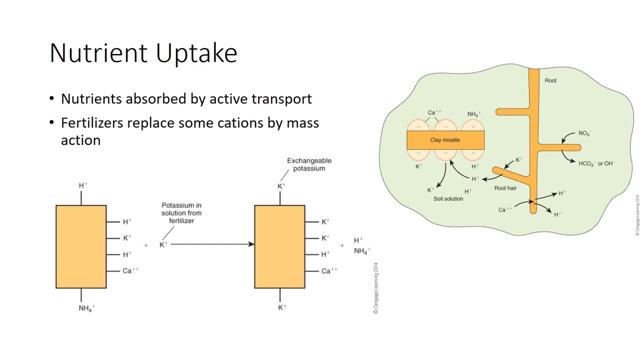 rhizosphere. When a grower limes or fertilizes the soil with a nutrient base, the base cation replaces other cations on exchange sites. due to the effect of mass action, New root tips must be constant. Roots are constantly formed. for efficient nutrient uptake, Root interception results. 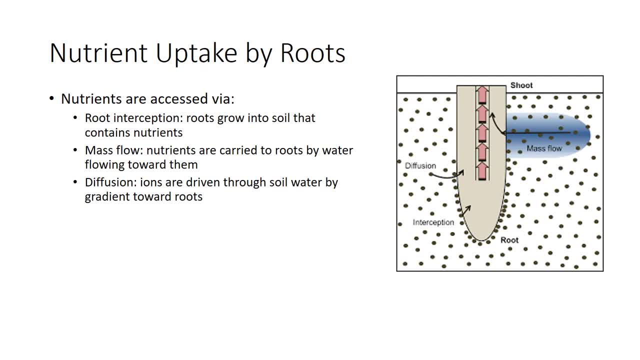 directly from the extension of root systems. As new roots grow, they displace a volume of soil that contains nutrients. Those nutrients are at the root surface and are readily absorbed. Mass flow carries nutrient ions to roots from nearby soil and water flowing towards roots.